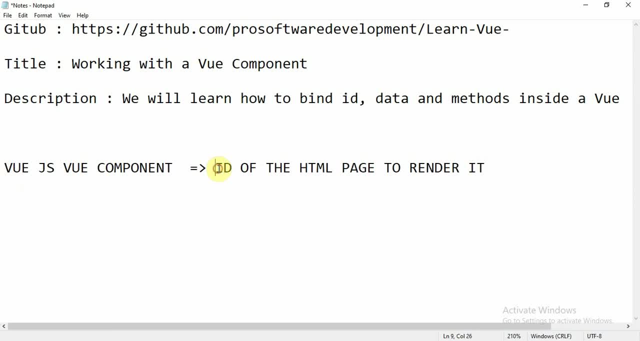 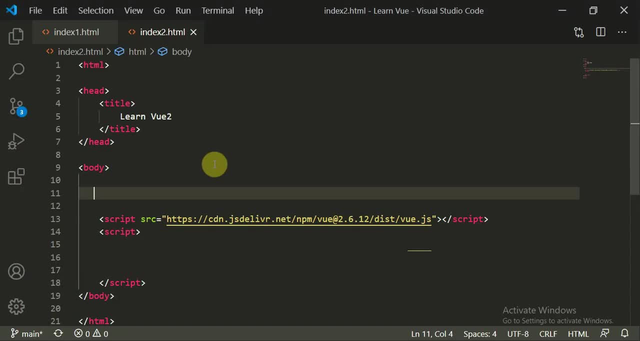 element, so it helps the view component to render on the html part using an id. so that's pretty simple now what you can do. you will create a new html page that is index 2.html in the previous on dot html, and you can add the view js script inside your it, inside your body tag. but make 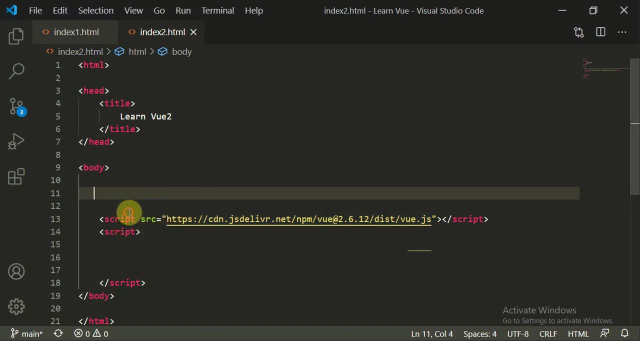 sure that it should be at the end of the body tag, not before it. so this makes like it will perfectly render everything. so the title is: learn youtube and we will give a create a view component. constant view, component 2. okay, i'll say constant view, component 2 is equal. 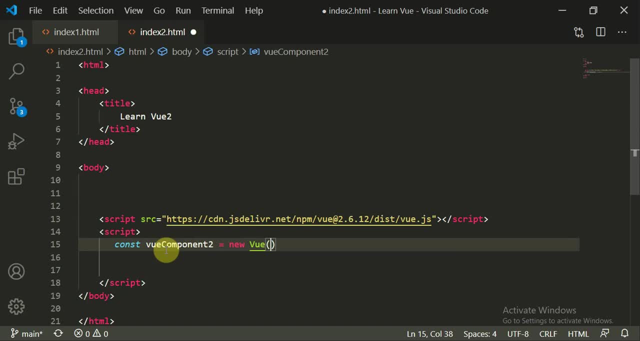 to new view. it will call the view constructor and the view constructor has a json object. perfectly fine. so now you can see it has a json object. now i'll what i'll do. i'll press enter. it has three things that are: element, which will have the id, and then it will have a data which will be in in itself a json object. 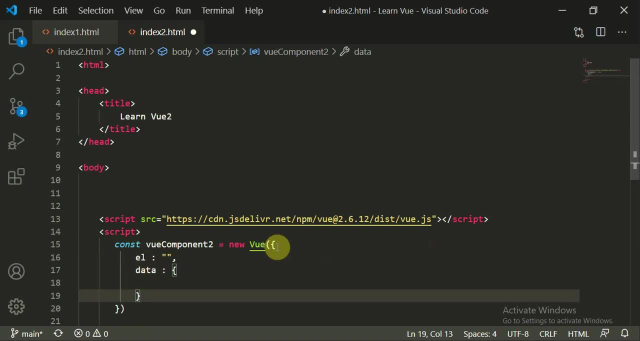 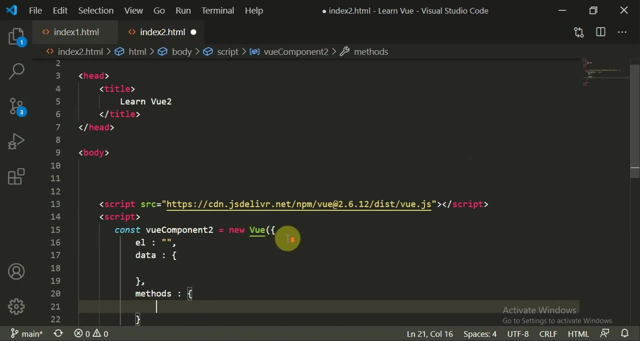 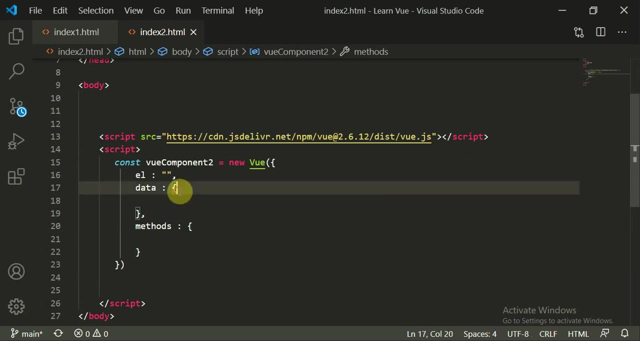 and then it will have methods. methods will be also a json object, so it will remember all those three, all these three things to put. you are perfectly fine with the your view component, so inside this i'll put: a counter is equal to zero and inside this i'll call the method. 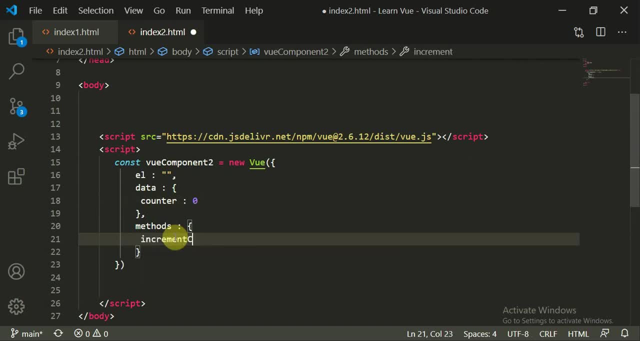 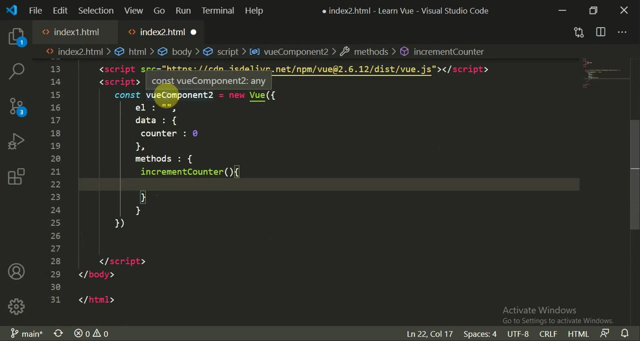 i'll call it increment counter. okay, and what i'll do? i'll call the method increment counter and, assuming, just for assuming, the case that forget this as a view component, delete it as active and create this as a class. so, if this is a class, if this is a 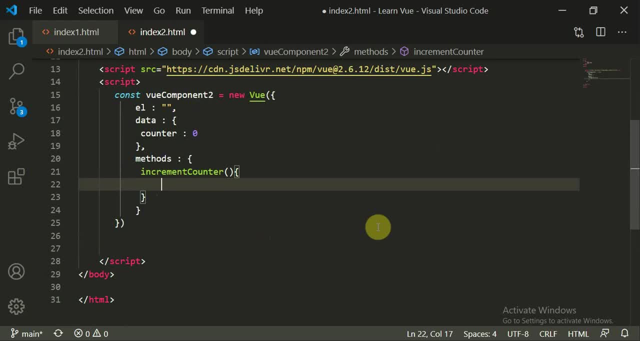 class. so what you can make: that if this is a class and if you want to access the data of this class, you can use the access this via this pointer. so this dot counter plus plus. so every time i click on it i'll increase the counter to to show this. i will increase. 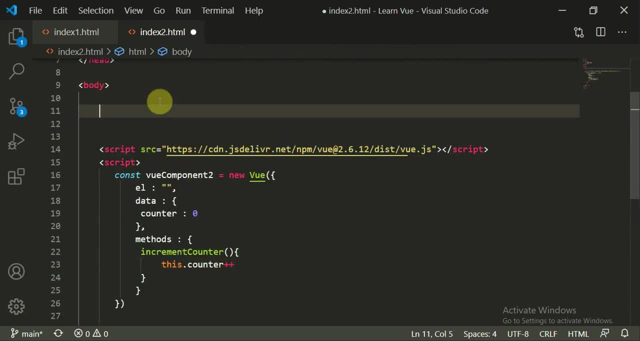 the counter to to show this as a view component. so this will be the view component and then i'll keep it for now and this will be the class type. ill make the data class then and then i'll the front end. what I'll do, I'll make a div. div id is equal to myapp2 and then 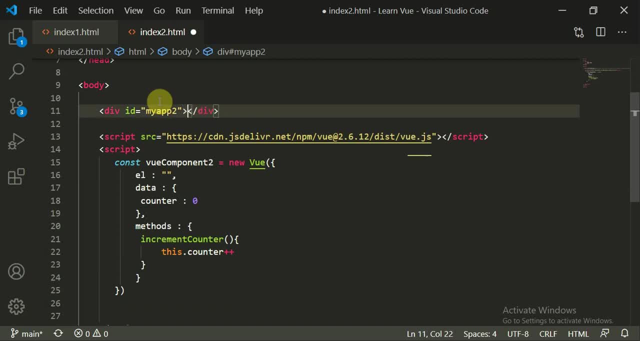 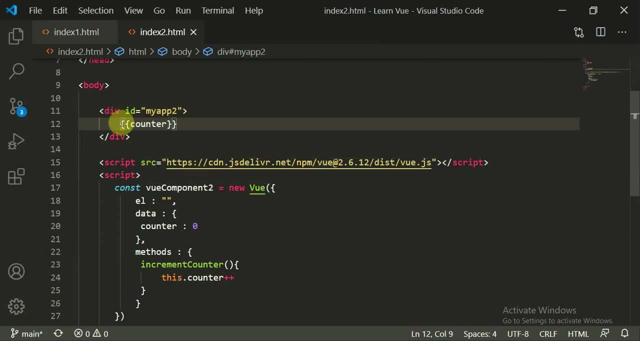 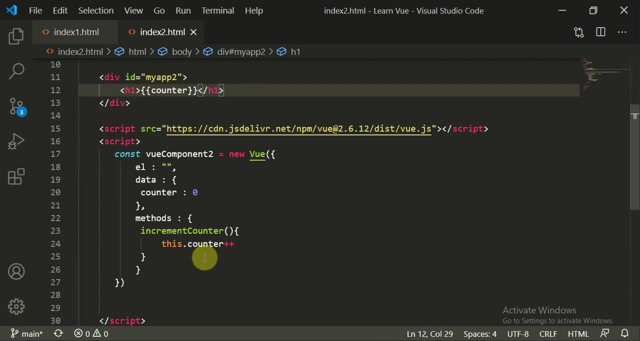 I'll close the div. perfectly fine, and what I'll do I'll. I'll create a counter variable using the handles and I'll give this as h1 tag. so I hope this is fine. now what I'll do. I'll what I'll do now, what I'll do. I have to refer this. 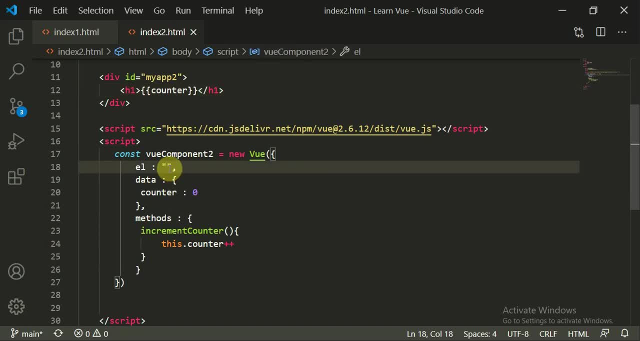 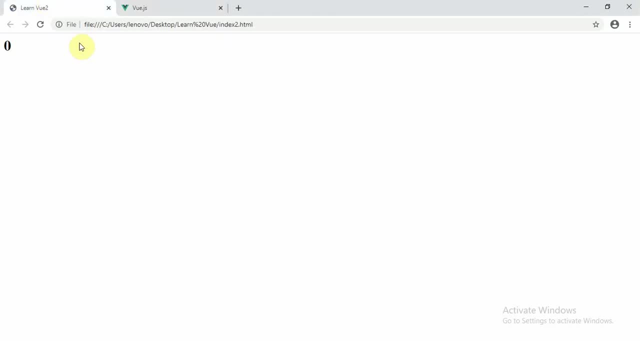 element to this id, that is hash myapp2. now I'll go to the page and I'll refresh this. it says zero as a counter. perfectly fine, but what does something happen on the click? nothing happens, because for this I have to define a click function and 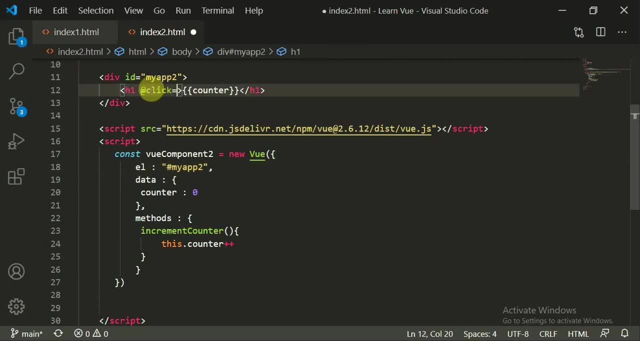 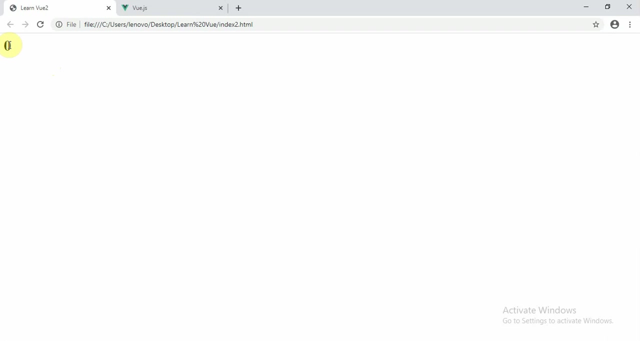 which can be defined even at the rate. click is equal to increment counter. so when I click on this, it will increment the count. I'll refresh this page when I click this. here you can see the count gets increased one by one, by one. so this is how you increment the counter by this function, that is, at the click at the rate. 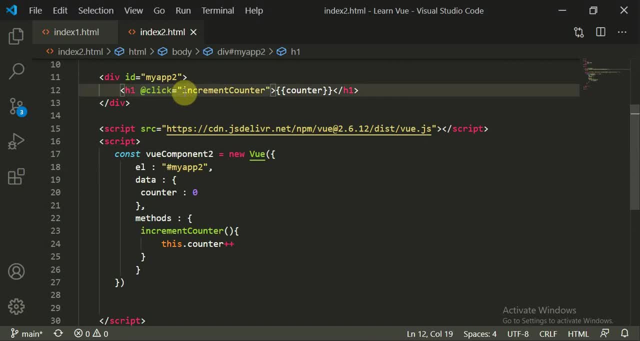 click function which Dec gloves offjamム do is the same the token and Bク berm Napca Makala e. sure you will do the same thing on the click-on click functionality as well. okay, now I will show you a small example. Let me add another thing that this text is. we'll do hello world. okay, now I'll show you a small example. let me try Another thing. that is: text is equal to hello, what that is Hello world, and okay, now I'll show you a small example. let me try Another thing. that is: text is equal to hello world. and what you can do. also, you can add: a flag is equal to false, or you can add it: a flag is equal to false, or you can add: a flag is equal to false, or you can You canанию for text to be, when I click on this word, what I'm typing inside. 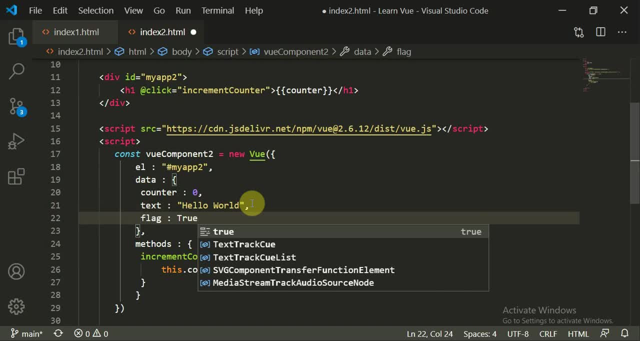 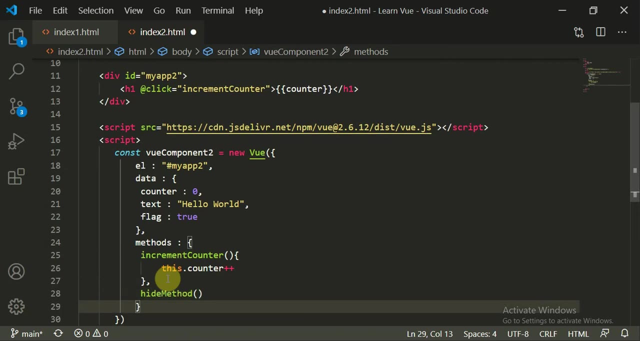 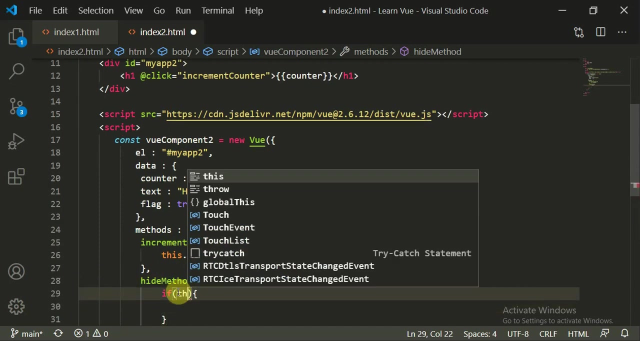 or you can click on flag is equal to true. so what you can do, you can call a method, hide, hide method and you what you can do, a hide method can will change this flag. okay, this if, if, the if condition here. it will change that if this dot flag is equal is equal to true. 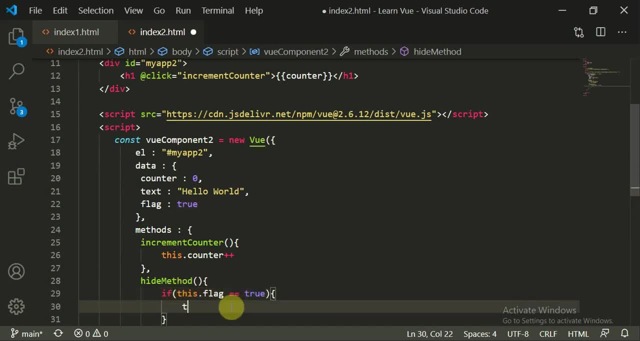 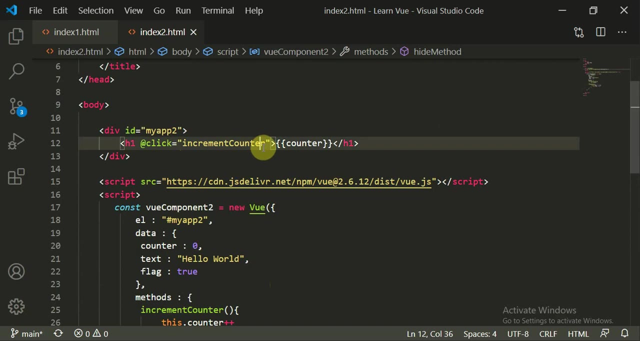 then this dot flag is equal to false. now this would change our flag. if this dot flag is equal to is equal to true, then this dot flag is equal to false. and how do you want to click that? you can change this to okay. first i'll show you one thing. i'll change this to text. 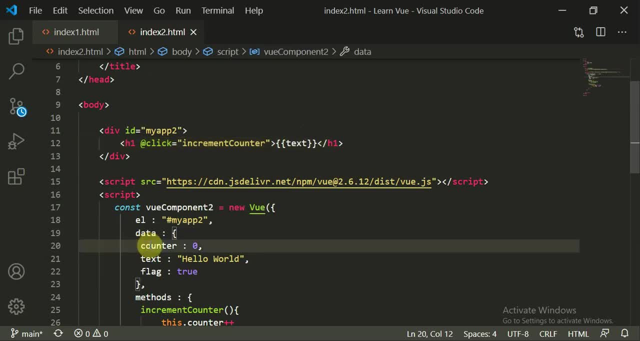 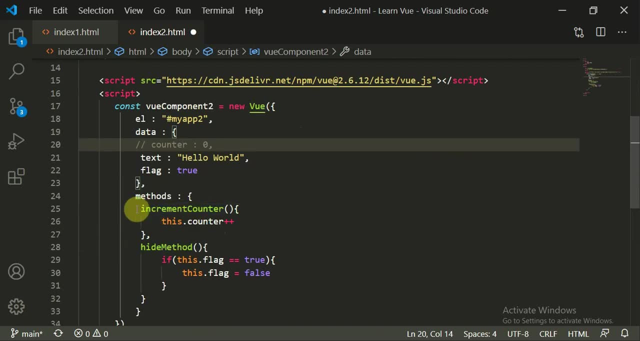 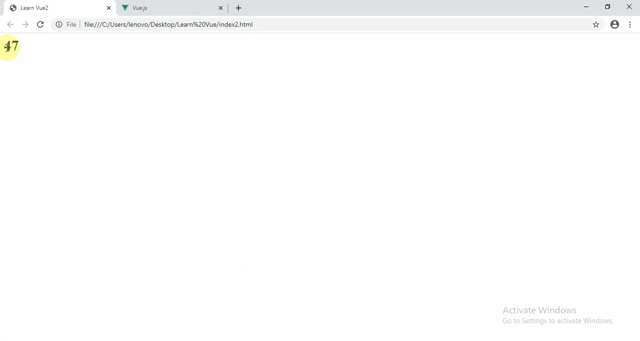 okay, perfectly fine, now what i'll do. i'll comment this out, so the this code remains as well, and okay, i think there is no need to comment, so let me remain this as it is. so when i refresh this page- uh, okay, this is the previous code working. so as soon as i click, the counter gets. 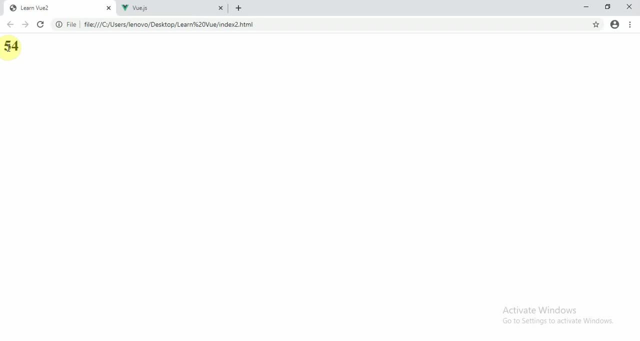 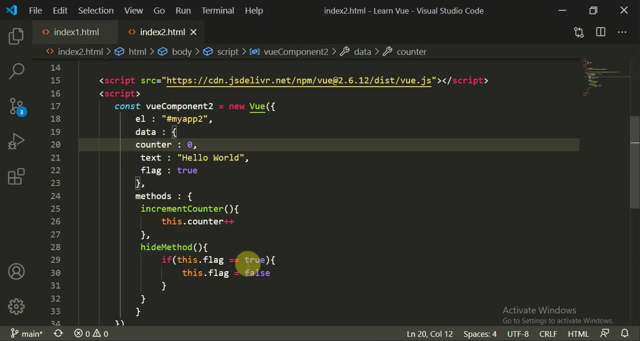 incremented. so this is the previous code working. when i refresh this page, the new code code gets added, split, so we get a text: hello world. but what i want to do? i want to hide this on click. so what i'll do? i click hide method. if this dot flag is equal to is equal to true, then this dot. 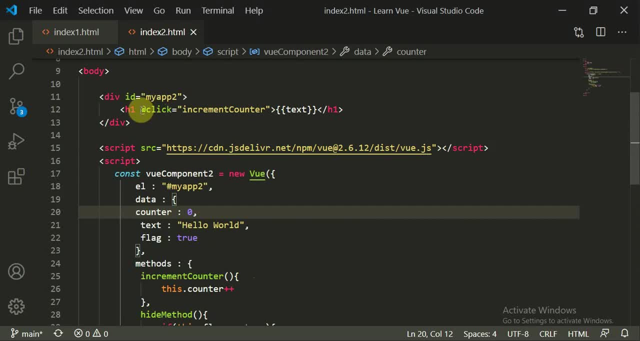 flag is equal to false. and what i'll do here that i'll do is that i'll do a hide method at the on at the right click function. i will call hide method perfectly fine, but i'll put another condition: that v if is equal to flag. 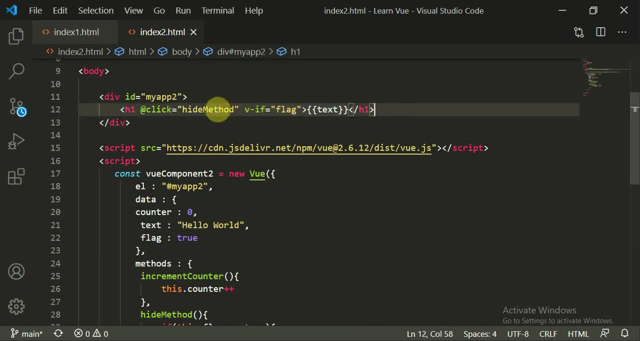 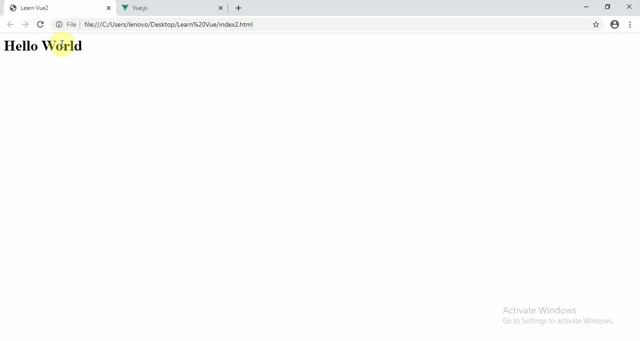 if this is true, then i show this heading, else i'll hide. else, if this is true then i show. okay, if it's false, then i don't show, and when this will turn into a chain it will turn to false when i click the hide method. okay, let me refresh this page. i click.